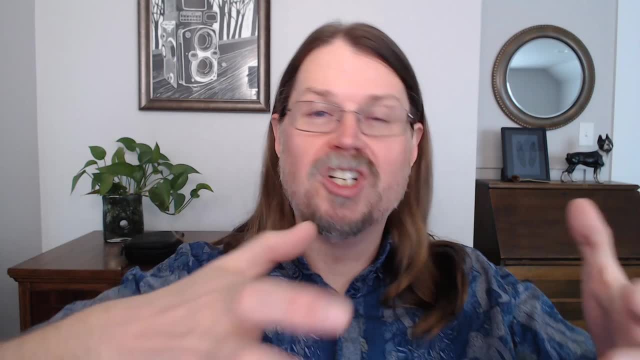 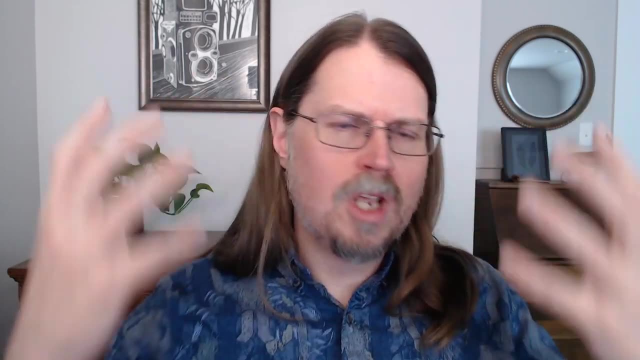 have a time component. So, for example, you grab a bunch of data about your customers from your database, let's say, and put it into Excel. Those customers are just, you know, like. they have static attributes like their name and where they live and how much product they've bought, and 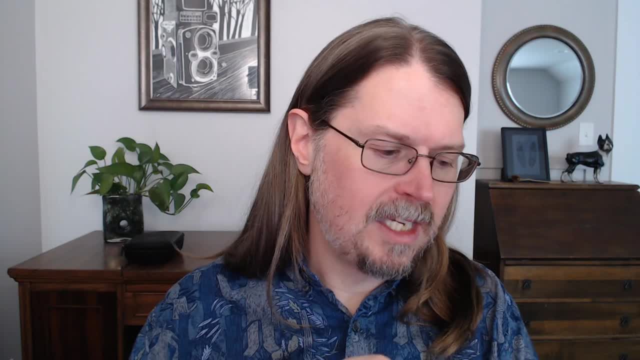 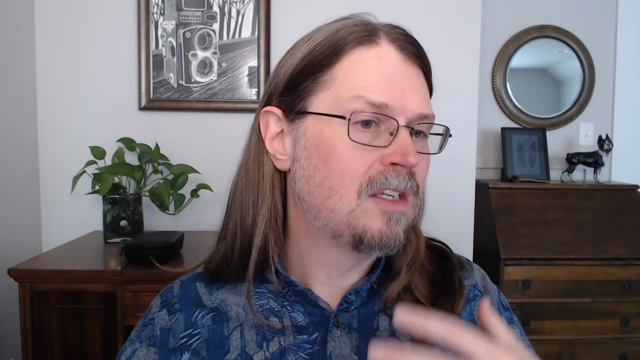 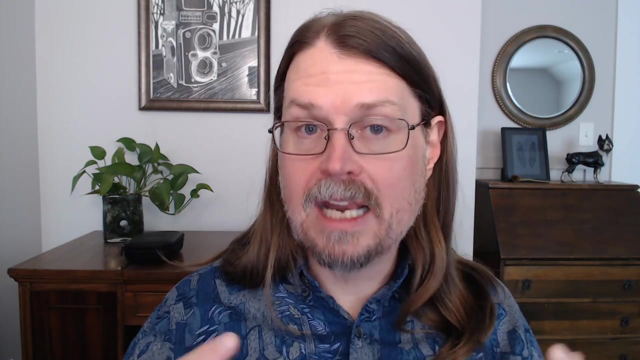 things like that. If you're interested in analyzing business data over time- so, for example, sales or expenses or your digital ad click-through rates or your conversion rates on your website, that sort of thing- I have a video dedicated to that. I call that KPI analysis and you 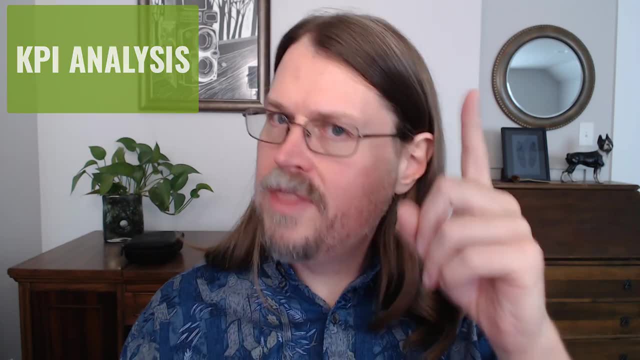 can find it on my website. So if you're interested in that, I have a video dedicated to that. You can just check that out up here, but don't click on it just yet. okay, It's there. at any point you say, hey, this video isn't for me, It's not what I really want to do right now. 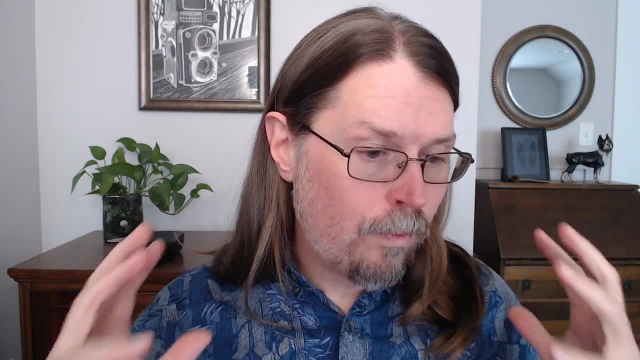 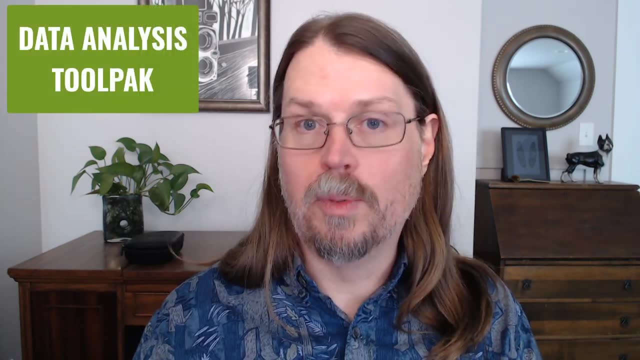 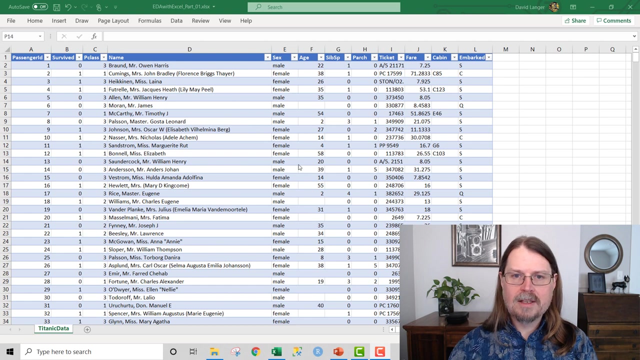 So there we have it. That's the housekeeping. So first thing that we need to do is go to Excel and enable something known as the data analysis tool pack, because that is super awesome. So let's go ahead to Excel right now. Okay, you can see here that I'm in Excel. This is the data. 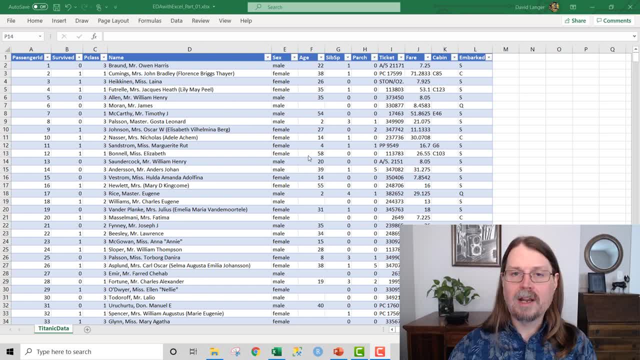 set that we will be using through the entire series, but we're not worried about that. What we want to do is enable the data analysis tool pack add-in in Excel, and this works for both Windows and Mac versions of Excel, If you have a modern version, if you have an old version. on 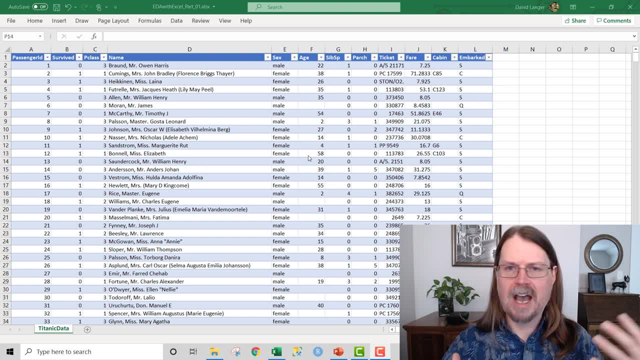 Mac, then it won't work. but if you have like 365 or 2019 versions of Excel, you should be good to go. So the data analysis tool pack is an awesome add-in that provides a bunch of really cool features for us to use to analyze our data, to explore our data, So let's go ahead and enable. 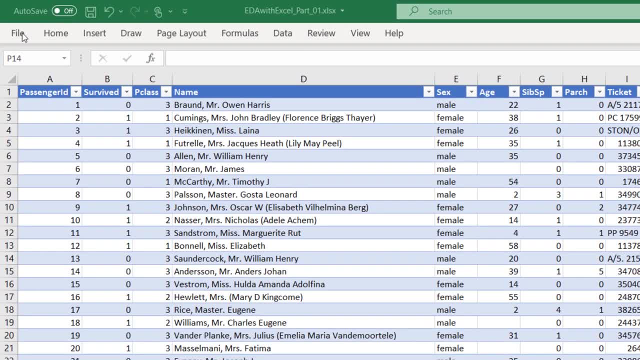 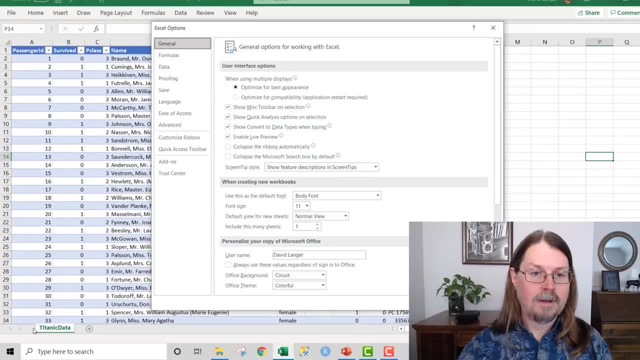 that. So how we do that is we go up here to file and we click on file And then way down here we want to go to options, And that brings up a nice dialog called the Excel options dialog, And what we're 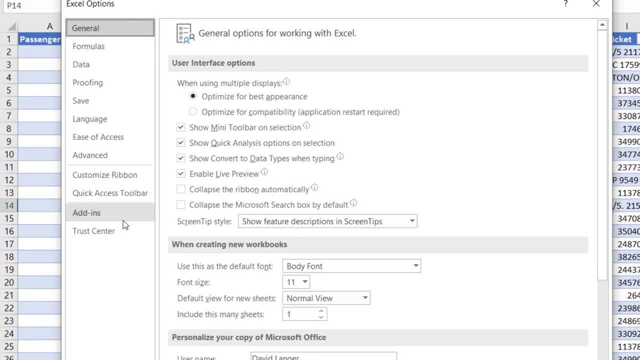 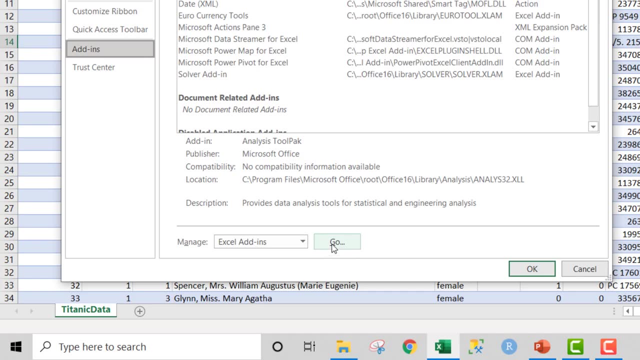 interested in is add-ins. So you go all the way down here to add-ins and click on that And we want to manage our Excel add-ins down here, So we're going to go ahead and click on go and that'll bring up a little dialog here And there's a bunch of different add-ons. 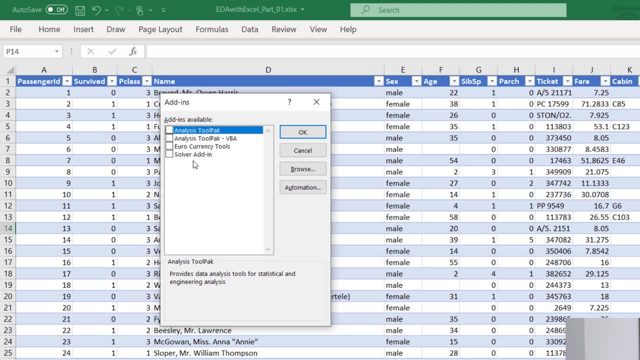 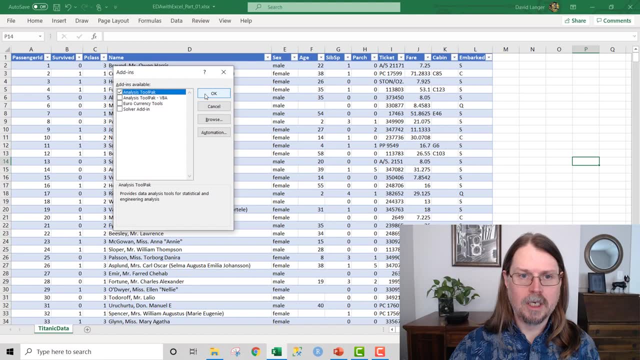 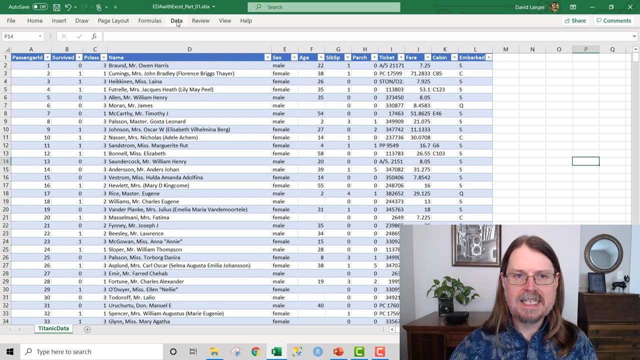 The solver is really super awesome. I might do some videos on that some other day, But right now all we're interested in is this first one here: analysis tool pack And click that, check the box there and then click OK. Now you don't notice a change, except for if you go to the data section. 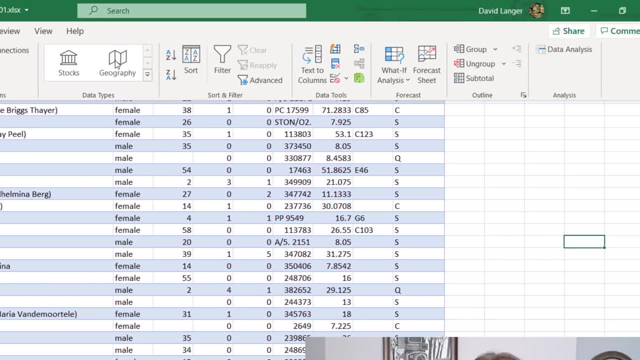 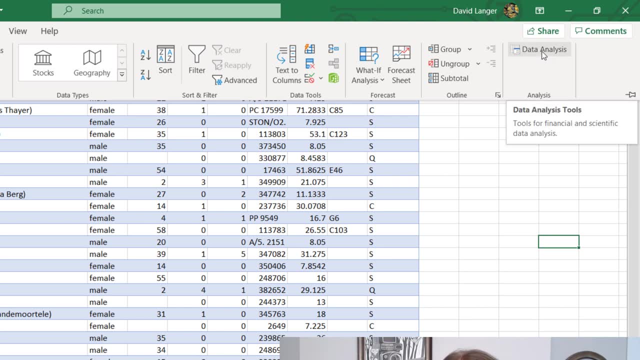 of the ribbon here, the data section of the ribbon, and click on that. You'll notice that way over here you now have a new subsection of the ribbon, of the data ribbon, called data analysis. That is the data analysis tool pack, And then you can go ahead and click on that And then you can. 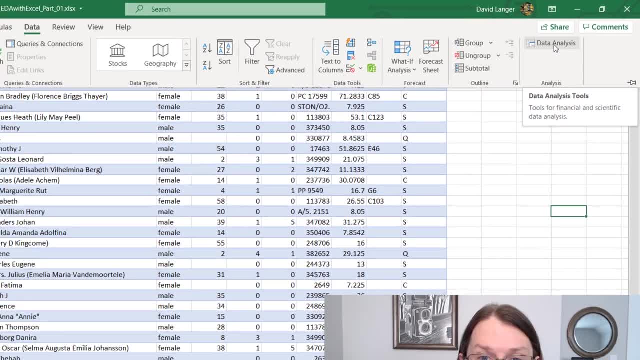 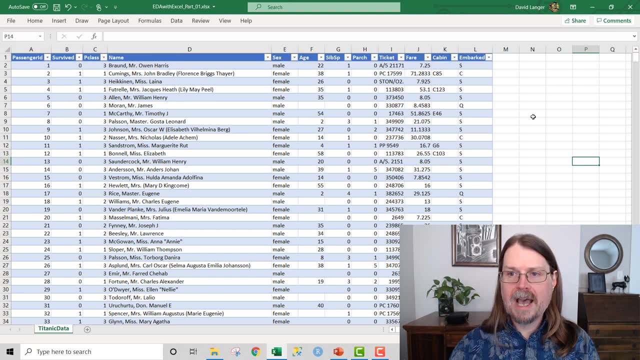 see that the data analysis tool pack is the analysis tool pack, And this is awesome. We're going to be using this in this video and we will likely use it in additional videos later on as well, So we've got the analysis tool pack open. That's awesome. That's our infrastructure. The 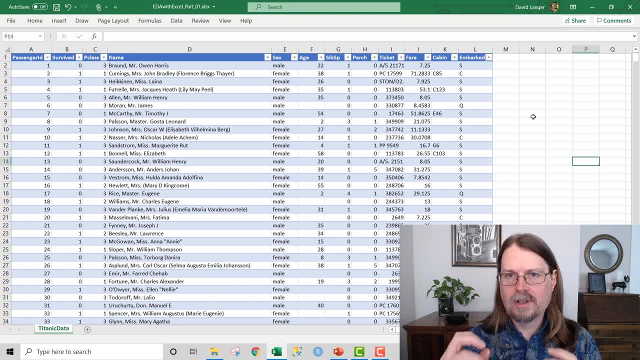 thing you have to remember is that the power of your exploratory data analyses are not a function necessarily of the tool that you use. We're going to use Excel in this video series. I also use the programming language as well. What you see here in this video series is the exact same thought. 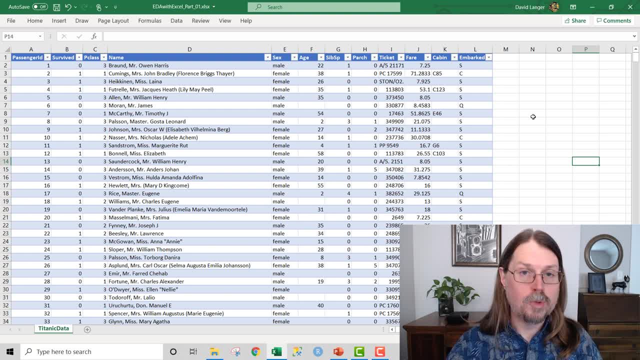 process and mostly the same techniques that I use when I use R instead of Excel. R just has some additional benefits that you just don't get in out-of-the-box Excel, but we'll talk about that at some other time. So the important thing is that you, as the data analyst, as the business person, 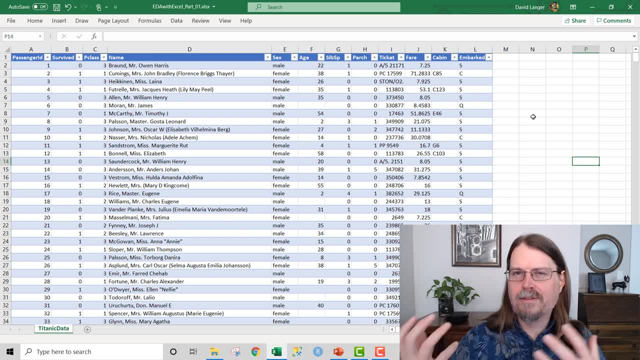 applying your knowledge of what's going on in the business and trying to figure out what the data tells you about that. that's the power of your exploratory data analysis tool pack And that's the most important thing. It's not the tools, It's how you execute the analyses, what you bring to. 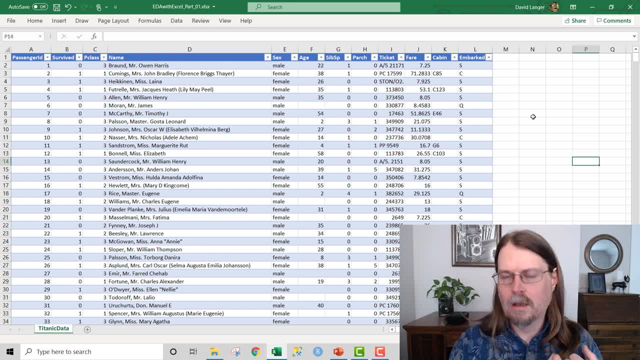 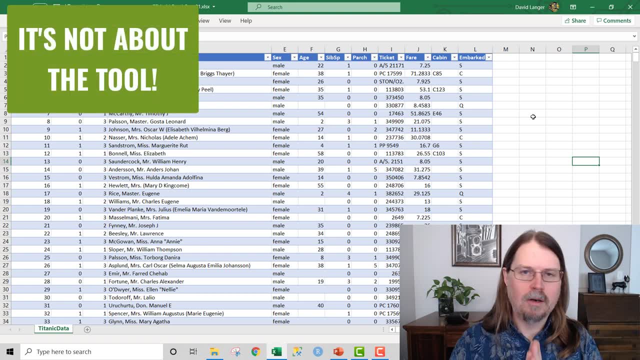 the table as the analyst. That's most important. And second, of course, is the data. If you have no data, there's no way to get insight. So those two things are most important. The tools doesn't matter. So what we're going to be focusing on in this video series is the thought process. 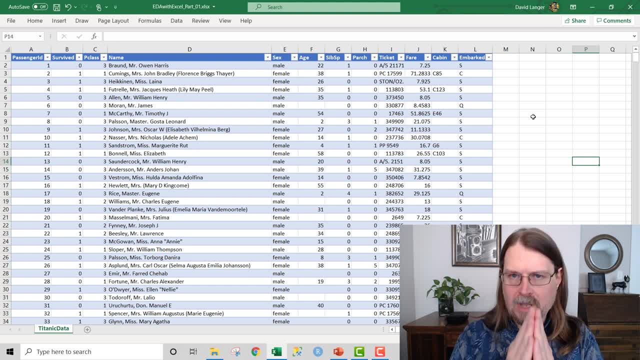 the ideas, the concepts, the kinds of analyses that we execute to derive insights from the data, rather than focusing on the tool itself. So you're going to hear me say this so many times throughout this video series and it's super, super important When you're using exploratory data analysis. 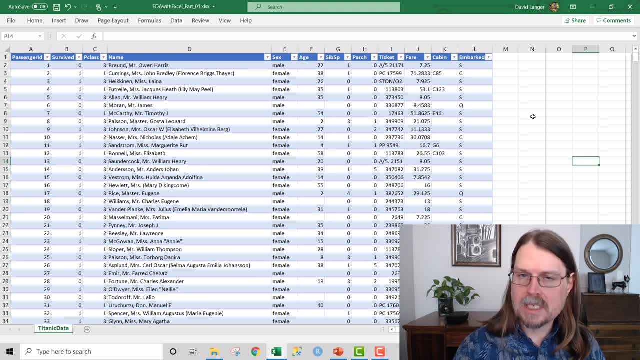 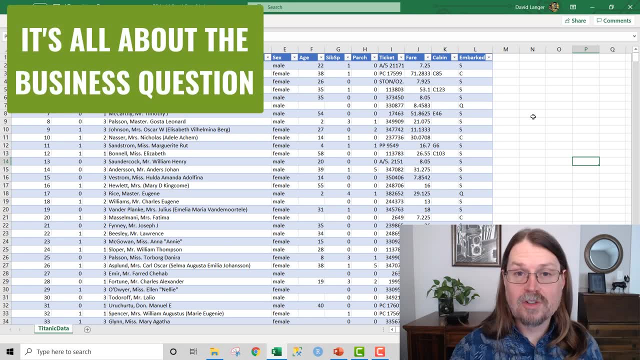 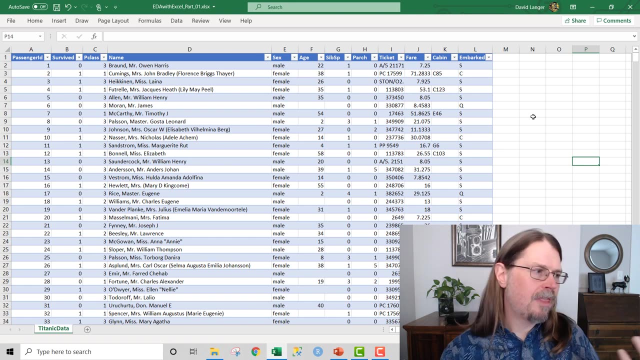 in the business analytics space. for analyzing business data, the single most important thing that you need to keep in mind is a question. If you want to use a fancy term, a hypothesis, but basically the same idea. you want to have a question. You can think of exploratory data analysis as this kind of this organic, natural. 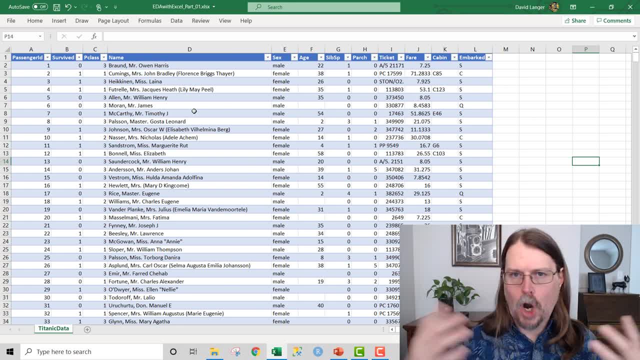 where you just sit down with a table of data like this and just start looking at it And you can do that. However, in business analytics, my experience has universally been that if you want to have maximum impact, you want to focus on a business question, first and foremost The business question. 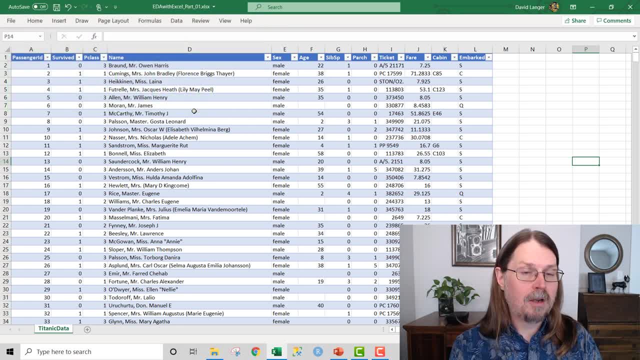 is the critical thing, And this might be a bit controversial, but I'm going to go ahead and say it anyway. If you don't have a business question, you should really stop and ask yourself: why am I doing this? data analysis, Business questions provide context. They provide ROI potential for 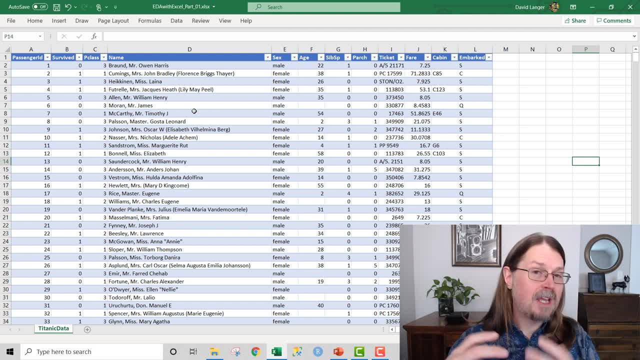 your data analysis. You should always have one, always- And sometimes maybe it's a business question that you want to investigate because it's related to another question that really interests you. So, for example, you're interested in understanding how your digital advertising 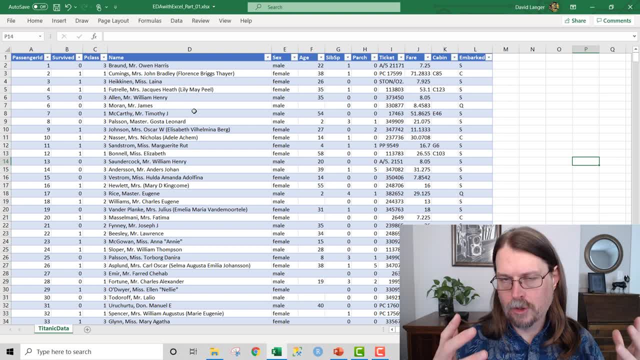 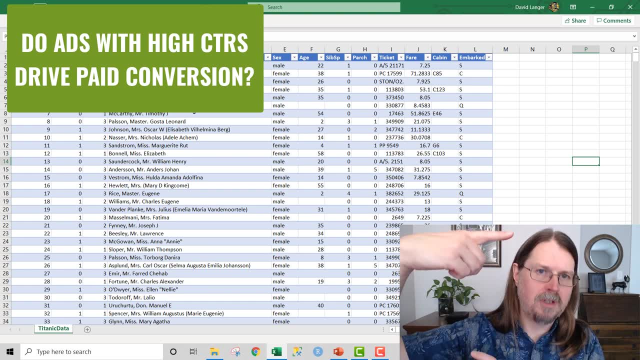 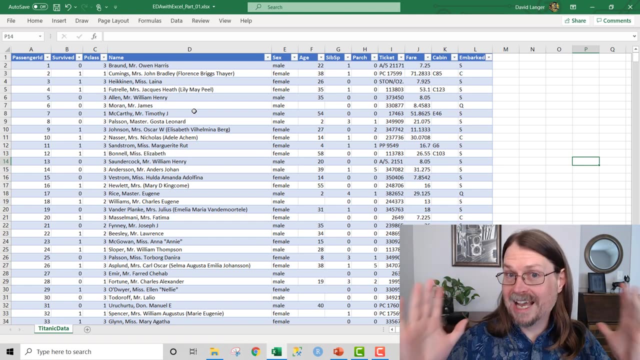 spend drives, paid conversions. So you might go then say, okay, well, what ads typically have the best click-through rate? That question, that sub-question, rolls up to the higher level question And that's okay. That kind of thing is totally reasonable and totally expected. First off, we got to start with our 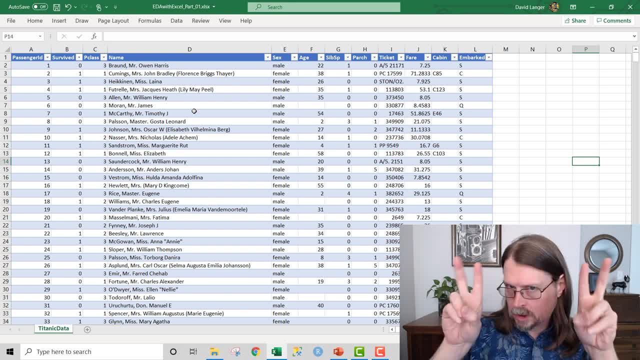 data set here and ask ourselves: what is the business question? I'm going to air quote that in this data set that we're interested in answering Now. this data set here is a very famous data set. It is the Titanic data set And I picked this data set. 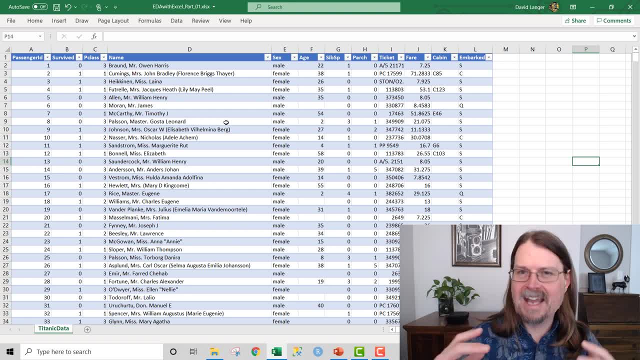 because it is a relatively small data set, but it's very interesting from an exploratory data analysis perspective. That's why I use this data set in all of my courses, all of my paid online courses, for example. It teaches you a lot about how to do data analyses. Some folks might be 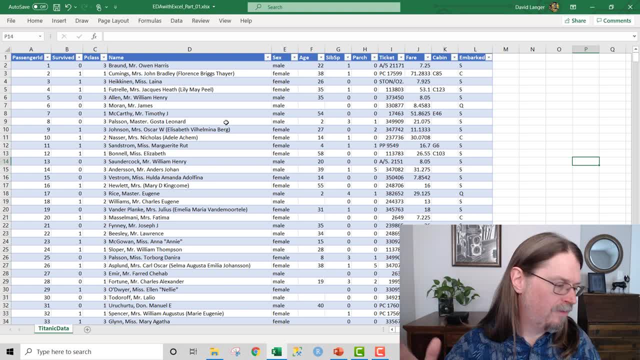 saying: well, Dave, why don't you use a marketing data set or a human resources data set or a finance data set? Those are all legitimate questions. The only problem is that those are all very domain specific. What I want to teach you is how to do data analysis, And I want to teach you. 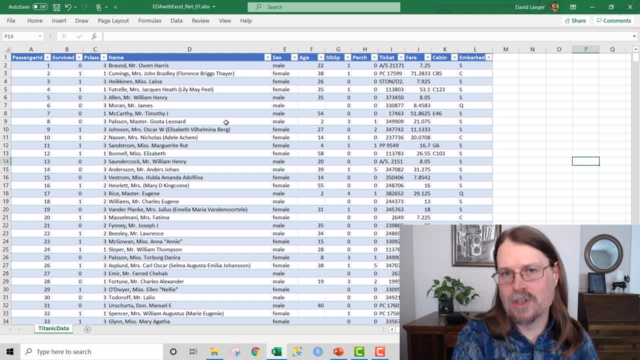 the general concepts that any professional can then take and use with their HR data or their financial data or their marketing data. So, not surprisingly, one advantage of using this data set- the Titanic data set- is that everyone's familiar with the problem, which is, unfortunately, 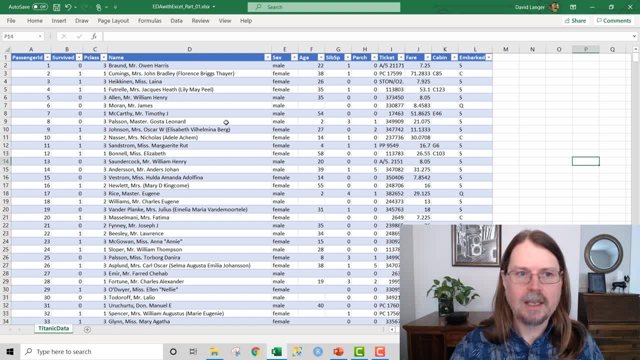 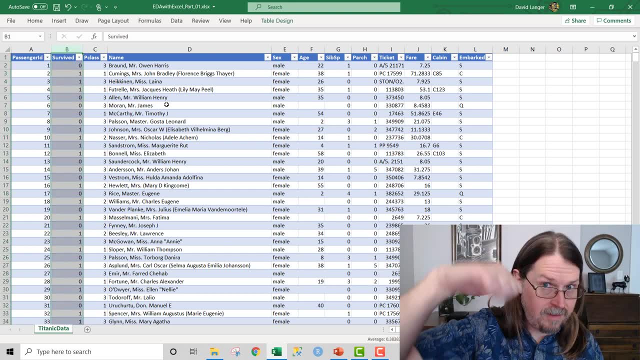 there were folks that perished on the Titanic And this column right here, the survive column- gives you a one if the passenger survived and a zero if the passenger didn't survive. So that's the one advantage of using this data set, The Titanic data set- is that everyone's familiar with the problem. 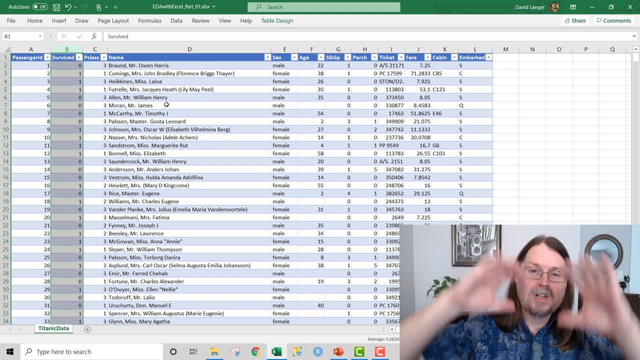 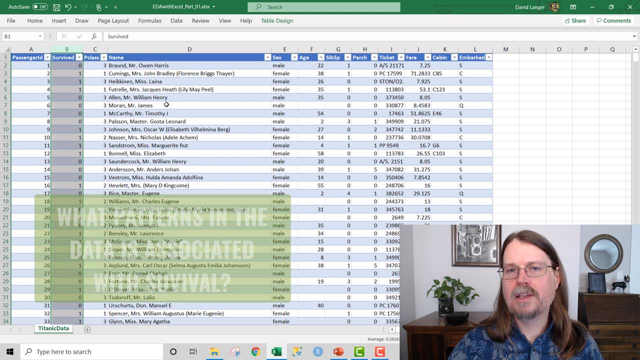 if they did not. So, not surprisingly, the high-level business question that we're going to be looking at throughout this tutorial series is: what pieces of data are highly associated with survival? That's the business question that we're going to answer, that we're going to try and 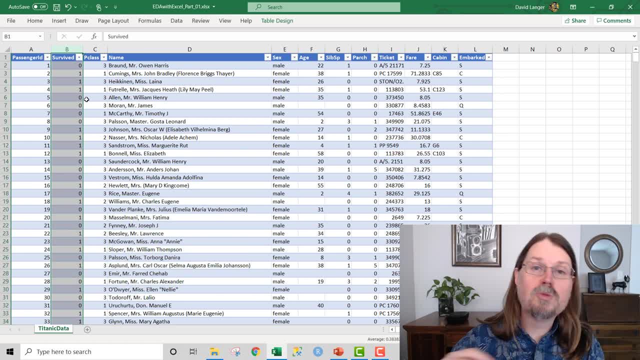 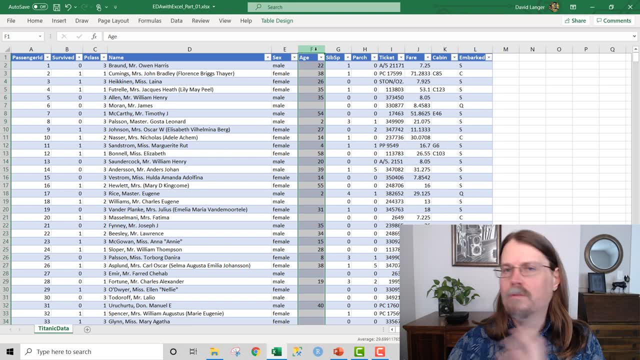 answer with our exploratory data analyses. Now, throughout the series, we might break down into a sub-question. For example, we'll take a look at age in particular later on, for reasons that will become clear later on, And we'll take a look at age in particular later on, for reasons that. 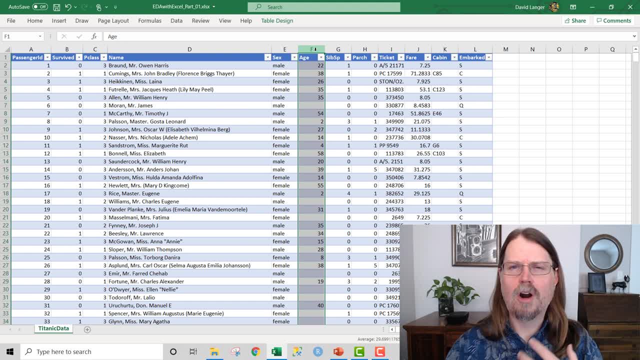 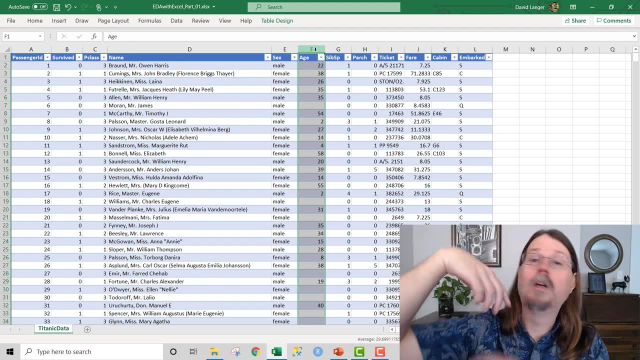 that will be like a sub-question: What factors are associated with ages? That's definitely something we're going to be interested in. That's a sub-question that then rolls up to the high-level business question of what factors, as evidenced by the data, are highly associated with survival. 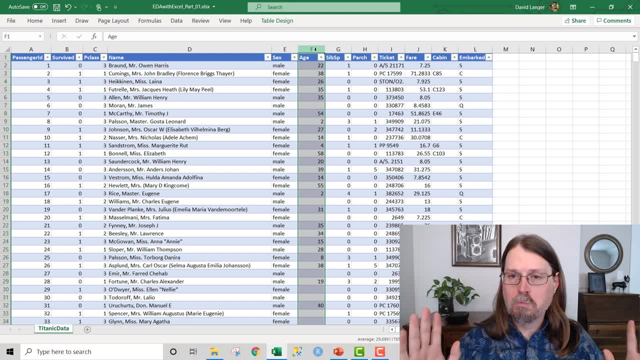 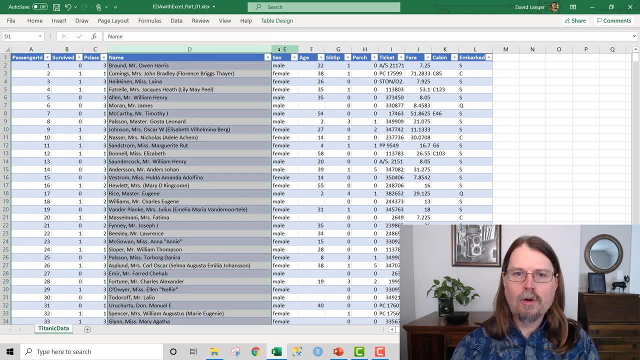 Okay, so now we have our business question. Great. First up we say: look, we've got a collection of data here. We've got, you know, some columns of data, And I'm not going to go through what any of these mean If you're already familiar with the data. 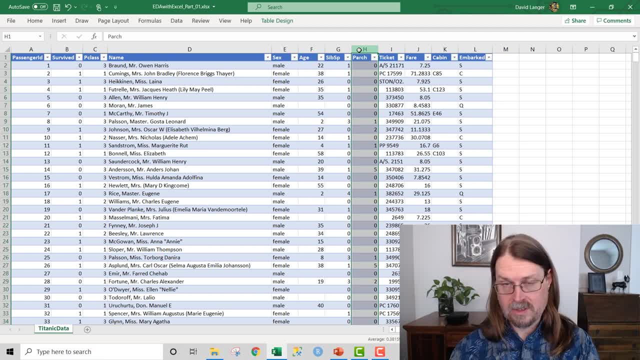 the data set and what they mean. that's totally okay. You're still going to get value from this series. If you don't know much about the data set, that's the best, because we're doing exploratory data analyses. However, one thing that we do know is that we want to understand how the rest of the 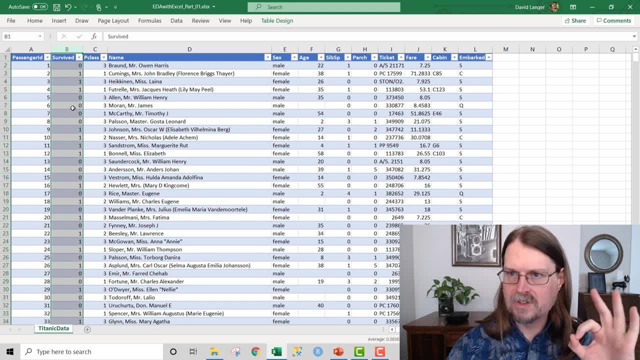 data in this data set is associated with survival. That's our overarching business question. that guides our analyses. So first up, let's just go left to right. Okay, we're doing exploratory data analysis. Let's assume that we can infer. 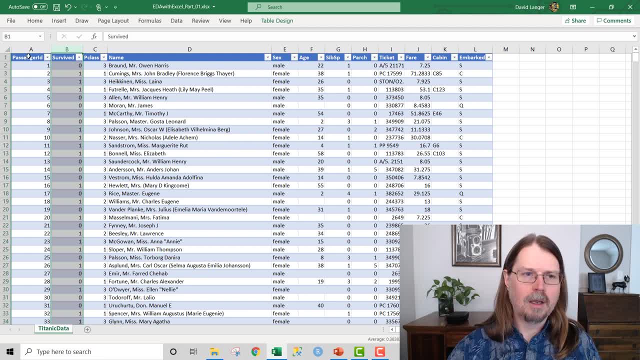 a little bit of what's going on in the data, just by the column names, the column headers. totally reasonable. You're going to see that all the time in the real world. So we know this is passenger ID. So if you're familiar with it, obviously if you're familiar with the concept, 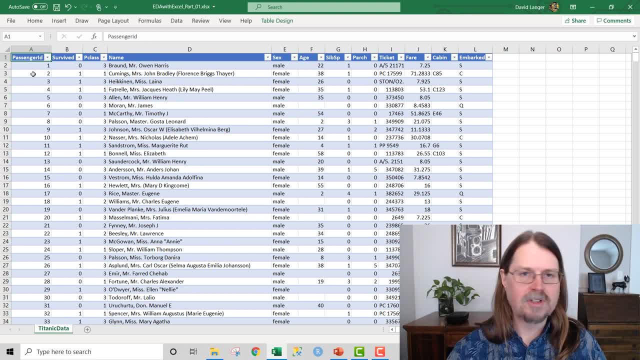 of an ID column. this is an identifier. So in the United States, for example, citizens of the US have an identifier. It's called a social security number. It's a unique identifier for each you know citizen in the United States. same idea here. 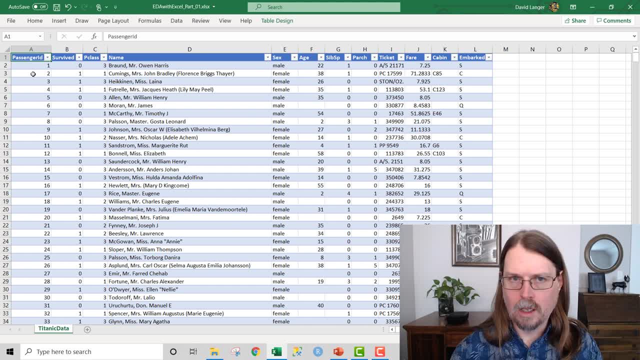 But if we didn't know that passenger ID was an identifier column, we could actually perform an analysis on this column and derive some insight And, in fact, the way I'm what I'm going to show you, you're going to actually understand why this column is likely an identifier. But let me 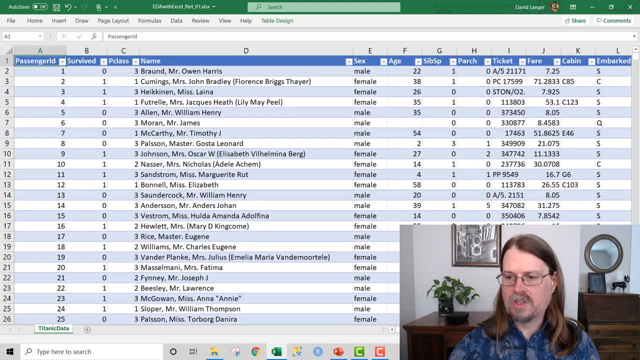 let me zoom in on the data first, So just so you can see a little better. So what we're going to do is we're going to take a look at passenger ID, column A, And we're going to do a very quick analysis on this column all up. We're going to explore it And we're going to do a very quick. 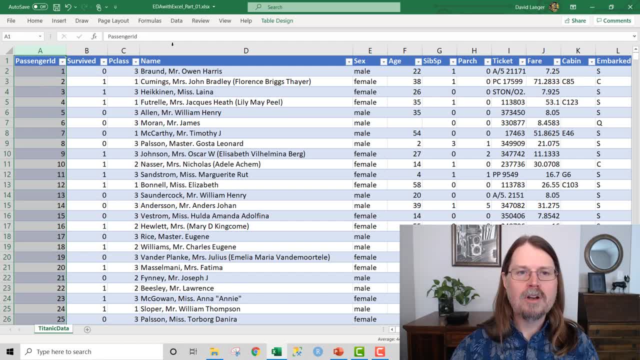 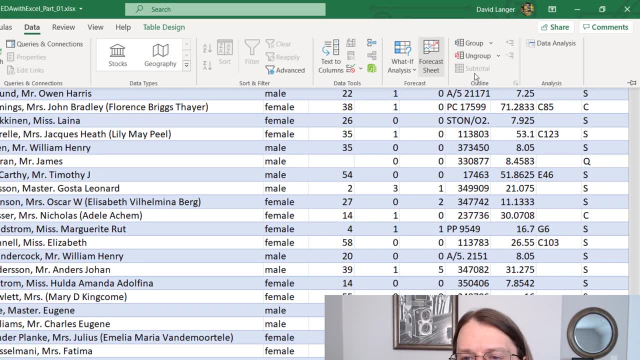 analysis on this column all up. We're going to explore it And we're going to explore it And we're going to explore it. And how we're going to do that is we're going to use the mighty analysis tool pack. So we click on data here in the data ribbon And we move over to the data analysis. 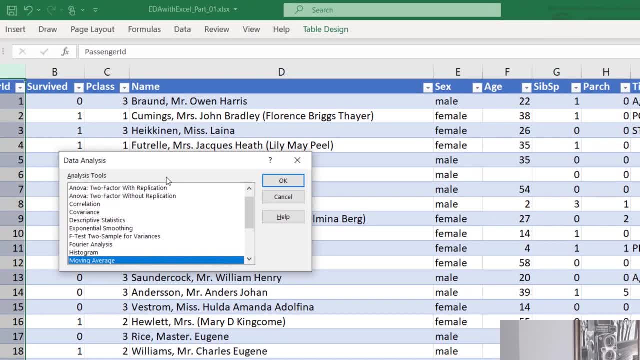 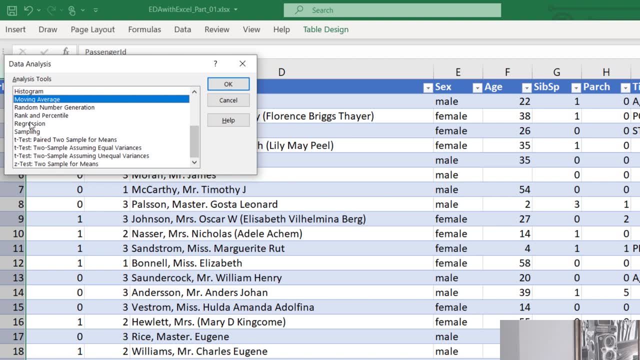 option here And we click that And that brings up dialogue And there's a ton of really awesome things that you can do with this. For example, you can do regression analysis. I teach a course that explains how to do regression analysis in Excel to folks with no technical background. 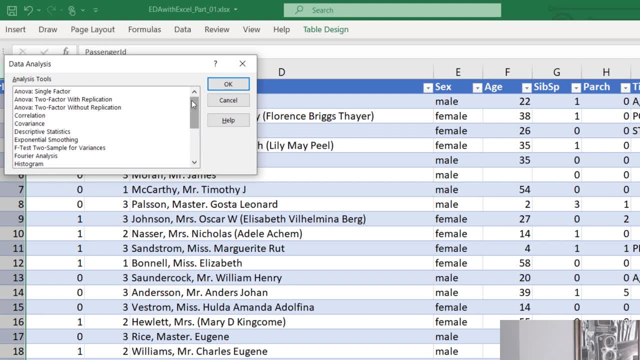 And I use this particular option. It is awesome, Okay, But for this particular analysis, what we're interested in is the descriptive statistics option, So that's the one we're going to select here. So we click on it, highlight it in blue, click okay And we get another dialogue And the 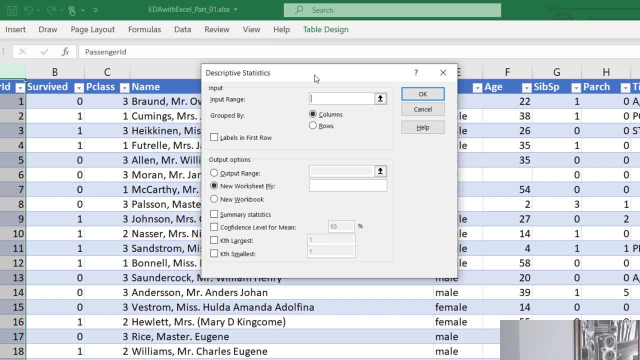 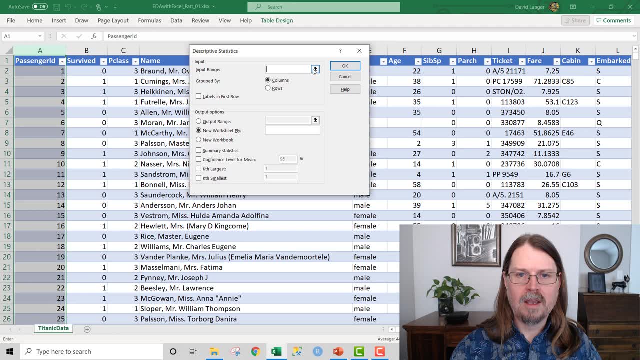 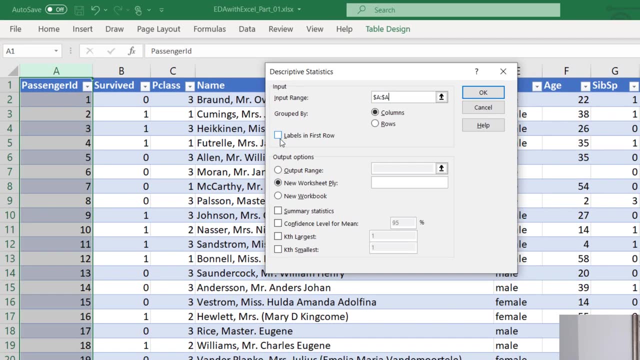 dialogue says: okay, you need to give me an input range. What are the cells of data that you want me to analyze with descriptive statistics? And what we know is we want to do column A, So we'll just do column A here. And then we know that we got a label in the first row, So we'll just go ahead and 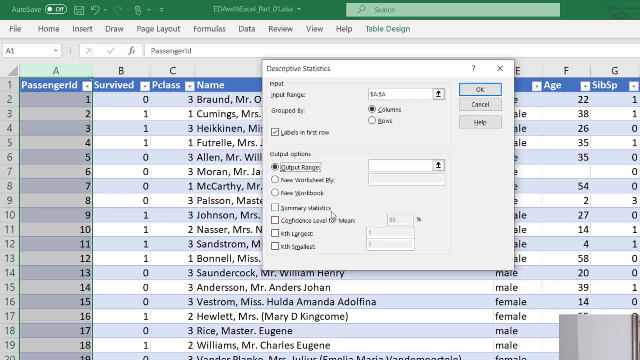 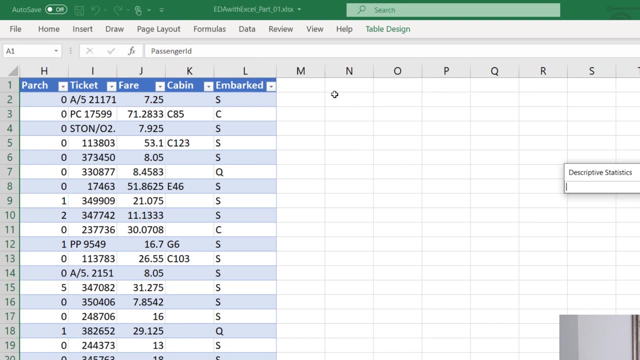 click that, And then we want the output in this worksheet. So let's just go ahead and go over here, Click the button there, And let's just go ahead and put it in N2, let's say N2.. That's where we're going to put it. 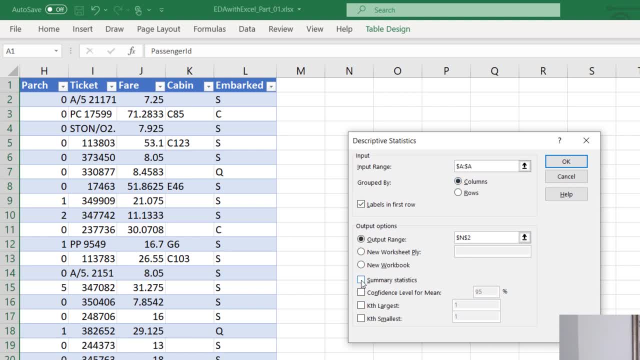 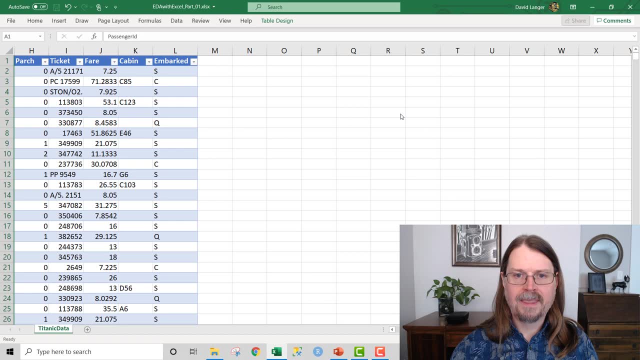 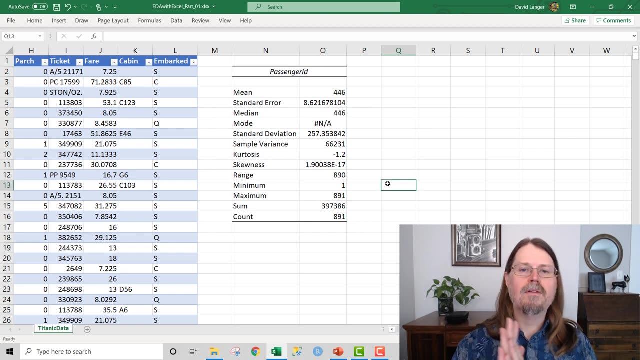 column a. we're going to do output range in two and then we're going to go and do summary statistics here. click, check that and everything looks good. we just click okay, and we chug away here and what we get here is some output for the passenger ID column, some descriptive statistics. 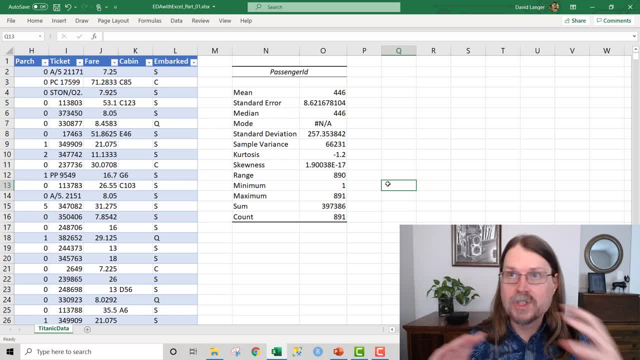 or summary statistics, and this is wild. the useful stuff. okay. so, first and foremost, what we want to do is take a look at the count of values, without even scrolling through the bottom of the table. what this tells us is that there are 891 rows, there are 891 values in the passenger ID column. 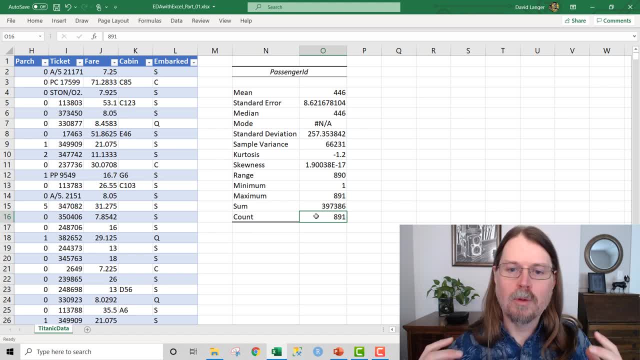 sweet. that's good. that gives us a lot of information about what's going on. how many pieces of data do we have? 891, excellent. so what we need to do here is then take a look at some of these other things and see what's going on. now. this is. 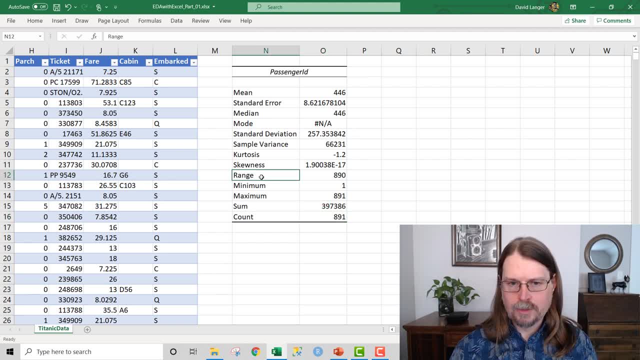 you. What next is interesting is taking a look at the range. The range is simply the maximum value found, and you subtract off the minimum value. This is super interesting because what this tells us is that, okay, we have 891 rows, we have 891 pieces of data. 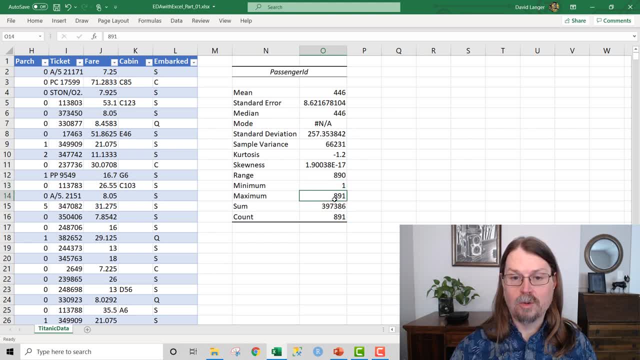 and the minimum value that we have is 1, and the maximum value is 891, and we have a range of 890 as a result, which tells us that, hmm, okay, this is kind of interesting If we had just a number, that was kind of random-ish. 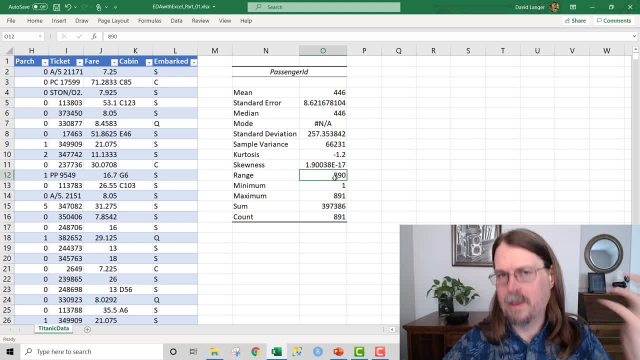 so something like revenue or somebody's age on the Titanic or how much they paid for their ticket, you wouldn't see something so closely associated with the raw amount of rows that you have. So if we scroll back over, what we can confirm here is that 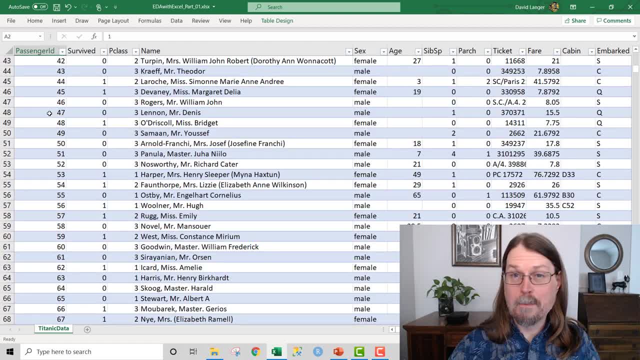 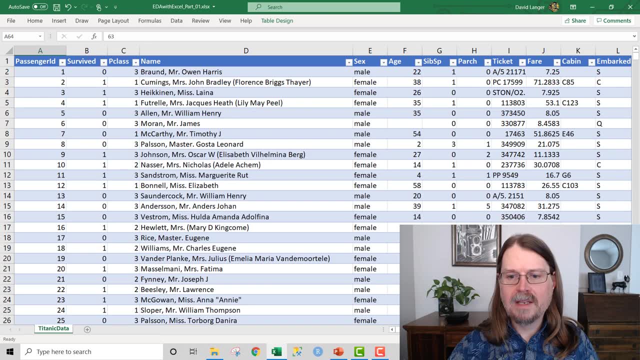 oh yeah, it looks like this is just what is known as A1.. This is a monotonically increasing number. Notice that we got 60, 61,, 62,, 63, so forth. Okay, but even if I didn't look at that, 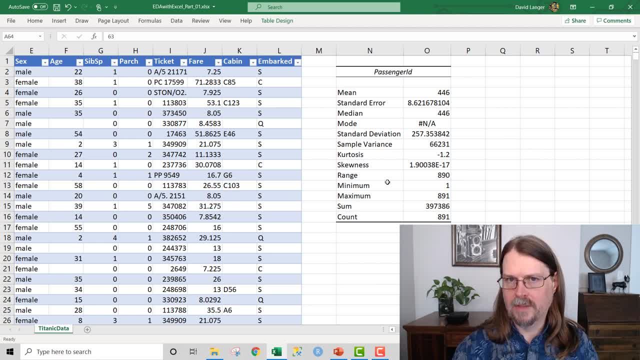 I can tell from this output here that there's something fishy going on in this data. It's unlikely that a typical numeric piece of data in business analysis is gonna have 891 rows with a minimum value of 1 and a maximum value of 891.. 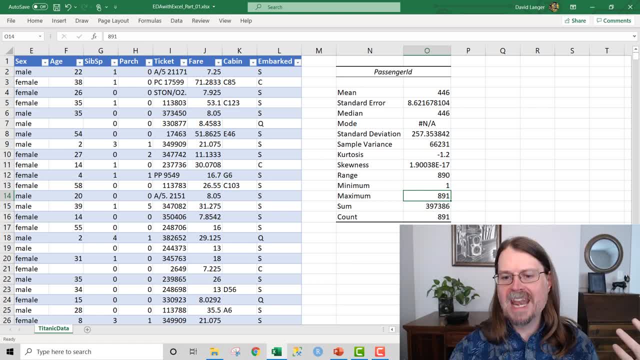 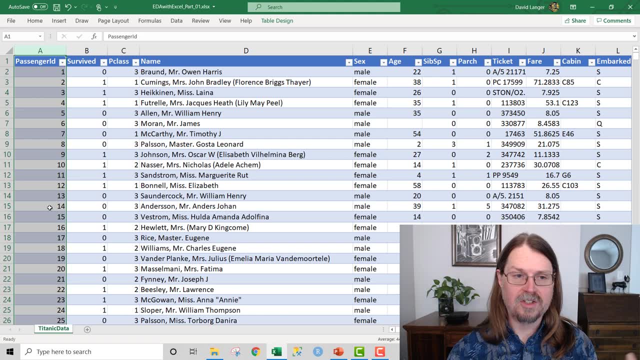 Okay, so that's interesting. Let's contrast this with another analysis. So we know this is a numeric column. It's not a useful numeric column, probably because it's just an identifier, but it's a numeric column so we can use this technique of descriptive statistics. 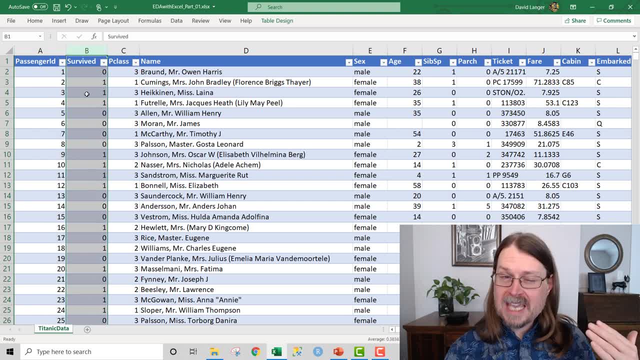 on numeric columns of data. Now, strictly speaking, this is encoded as a numeric column. It's ones and zeros. However, we know a priori- it's part of our business question- that in fact, this is actually not really a numeric variable. 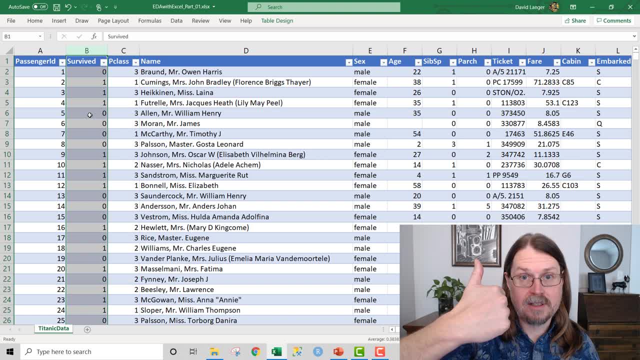 because it's simply a yes-no. Did the person survive? Yes, they have a one. If the person perished, unfortunately, then it's a zero. So we know that this is actually a categorical piece of data. It's got categories: survival or not survival. 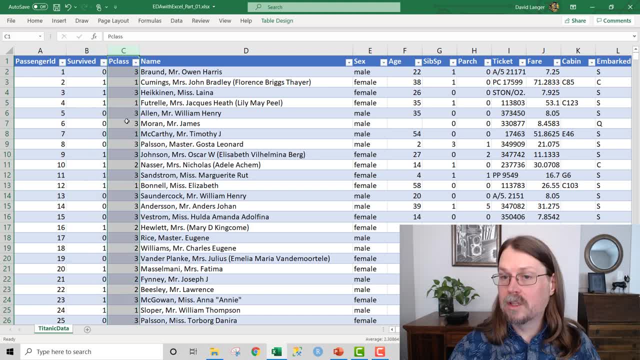 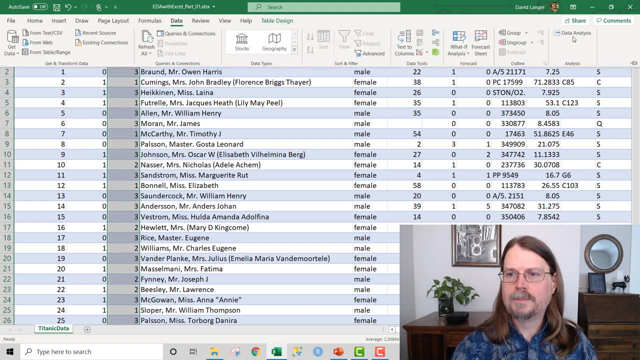 It's not actually numbers. We can take a look at this particular column of data now and let's do an analysis on that, on pClass, and kind of explore it and see what's going on. So once again we go up to the ribbon. 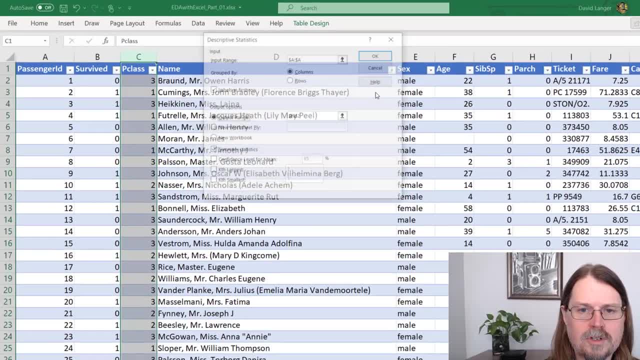 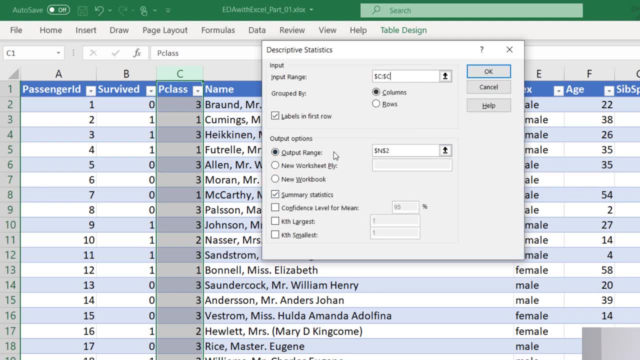 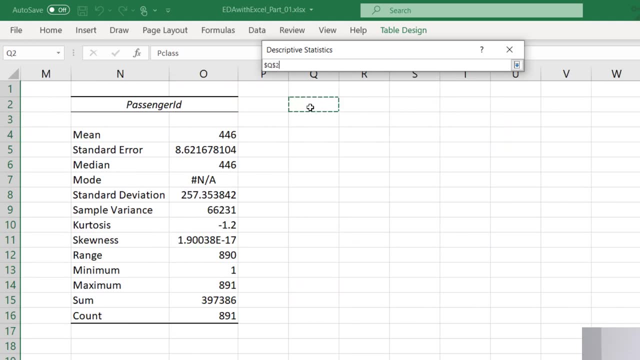 We fire up the data analysis tool pack, We want to do descriptive statistics. This time, though, we're gonna go ahead and click on column C here, And we're gonna change the output range and keep everything else the same, And let's go ahead and put that in cell Q2, let's say: 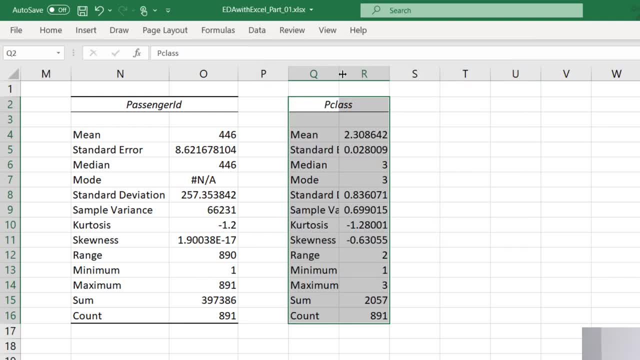 Let's start the output there And let me click OK. And then we've got pClass OK. So once again we've got passengers, Yet again, 16 judgement. That's one way to use pClass, All right. 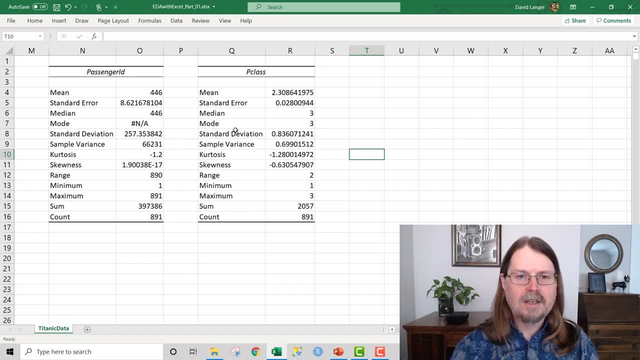 Yeah, So each one has a different ethanolic number in answering controls and there's three different outputs you could enter if you're looking, sense looking orЬ something interesting going on here. So notice that we've got a mode. Notice that over here. 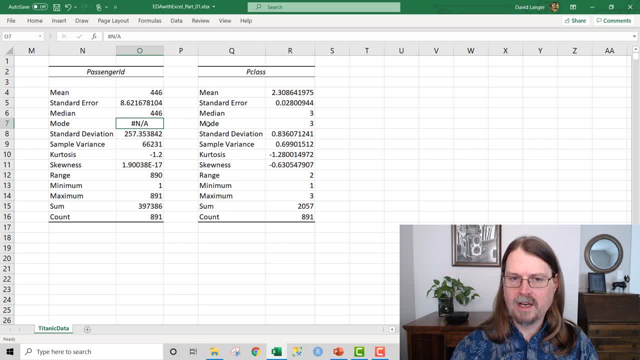 the mode didn't really exist, It couldn't be calculated, And if you're not familiar with the mode, is is it says: look out of all these numeric values, which one is the most frequently occurring And notice that this one is a mode of three, which is interesting because 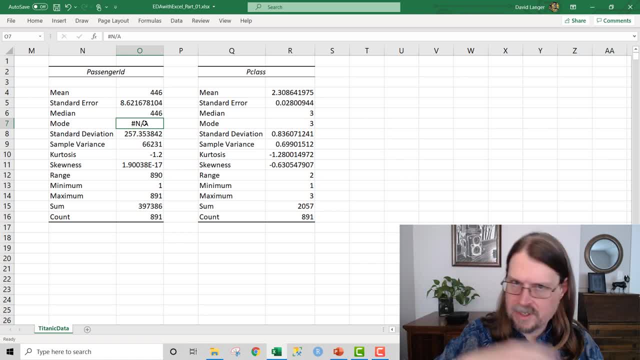 notice over here. we couldn't calculate it because every piece of data was different. Every piece of data was different, right, It was 62, 63, 64, 65, 66. There wasn't any value. that happened more often than any other, So the mode couldn't be calculated. but notice over here that 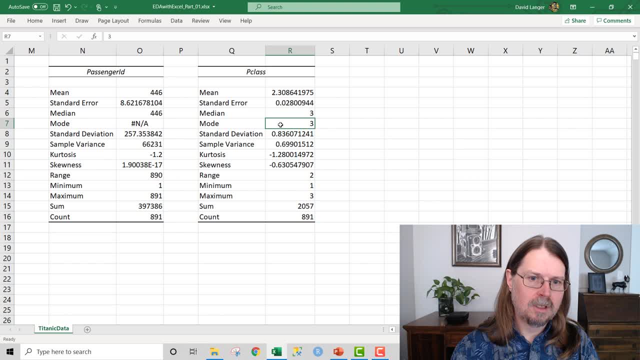 it can be calculated. That's really interesting. And then, if we go once again, we say okay, there's 891 rows, Great. And we say, oh, look at the range. The range is two and we have a minimum. 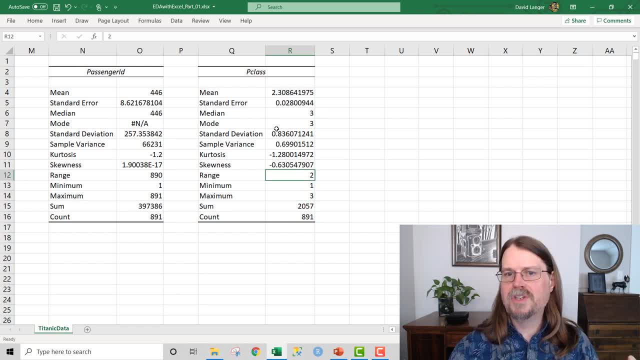 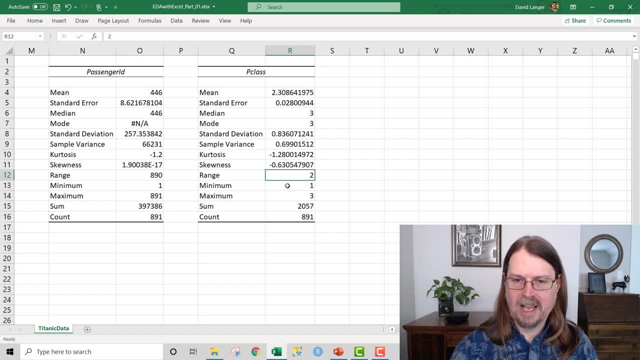 similarities between P class and passenger ID in terms of the range of maximum value. right That they seem to be well-defined, But notice that a big difference is that mode is not calculated over here because every value is unique, Whereas over here we say, oh no look. 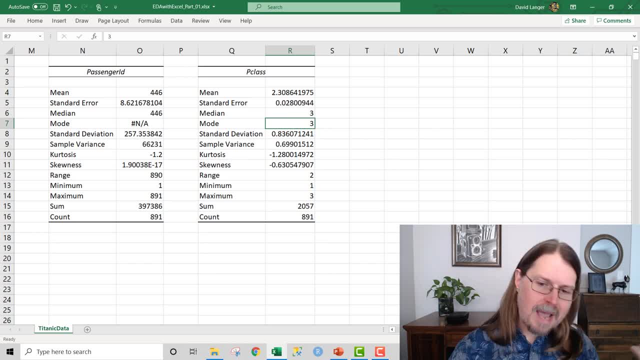 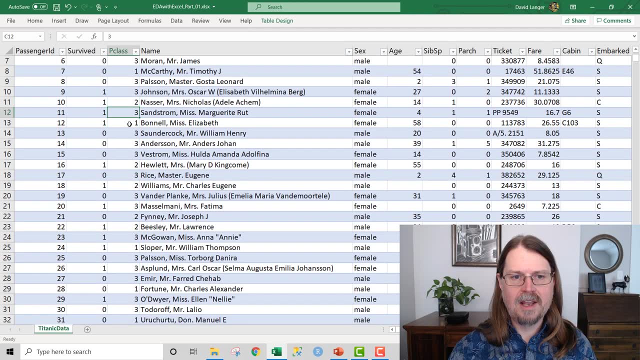 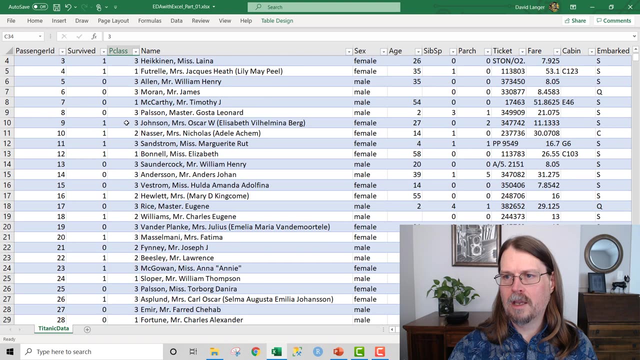 three is by far and away the most common value. So if we scroll back over to the table and just eyeball it, what this tells us is that this is a number column, To be sure, the way it's encoded. but maybe it's not really a number column, because what it's telling us is that we have a small number. 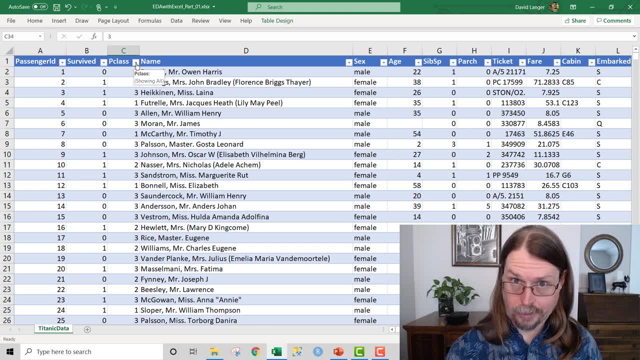 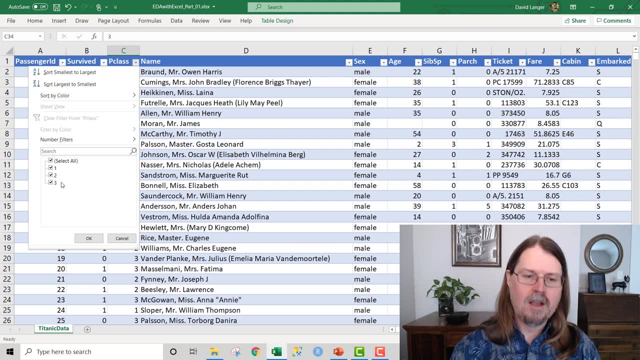 of values, And the easiest way to do that, of course, is also to check the filter in Excel. You just click on that and you say: okay, I've only got three distinct values available in this thing, So that's probably an indicator that this is actually a categorical variable, which kind of 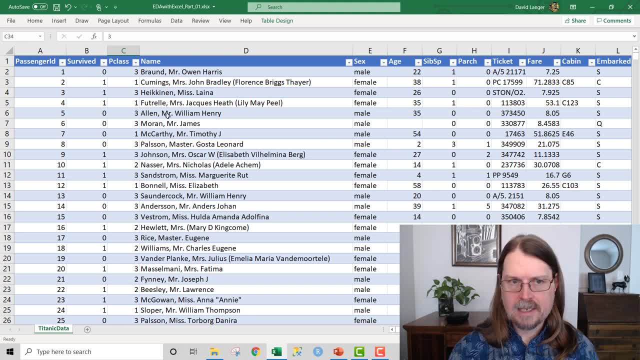 makes some sense if we think about the context, which is: this is the Titanic data set, and the P class probably represents the number of values that we have, So that's probably an indicator that makes some sense. What class of ticket did the passenger have? First class, second class? 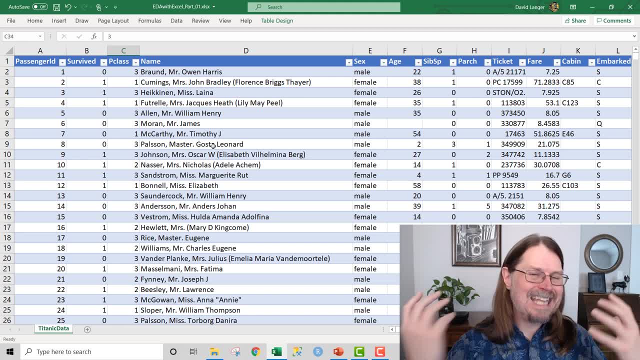 third class And notice how I didn't need the data dictionary, I didn't need a business subject matter expert to tell me what this means. I can use these techniques and just a little bit of knowledge about the data to kind of infer, maybe, what's going on. And that's kind of the heart. 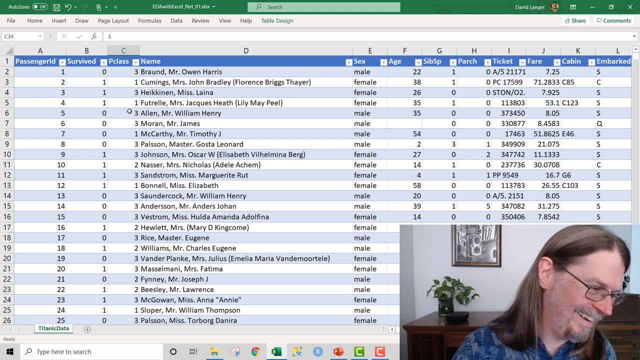 one of the hearts. one of the hearts, Okay, One of the ideas. how about that of exploratory data analysis? Next up, We're not going to look at name, obviously, because that's not numeric. We're not going to look at sex. 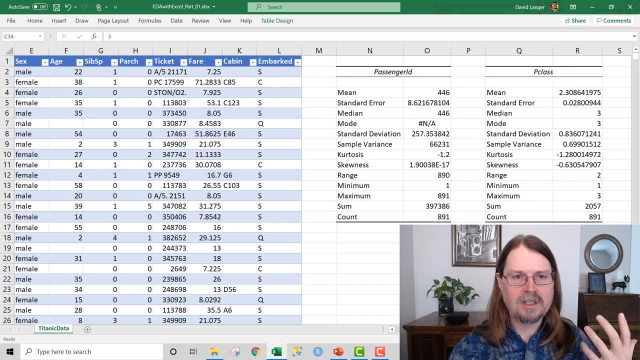 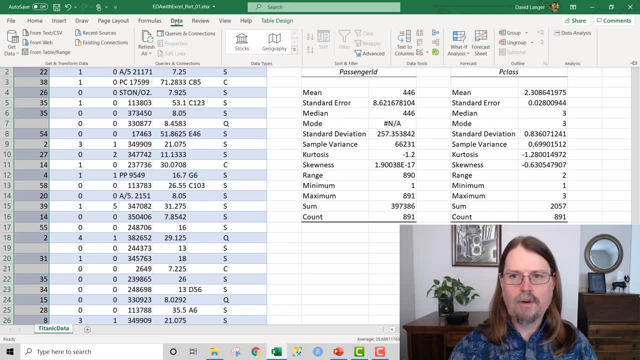 because that's not numeric. Let's take a look at age. That's probably a pretty interesting thing for us to look at. We're going to go and look at the age column here, column F. So once again we'll go up to the data ribbon here. We'll go to the data analysis tool pack. We'll click on descriptive. 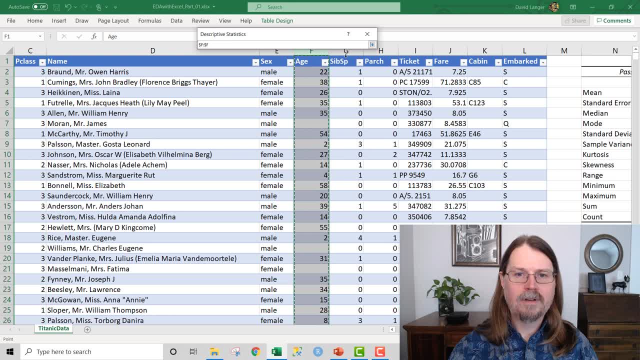 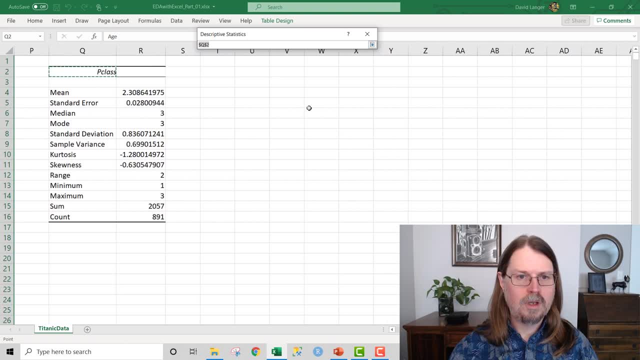 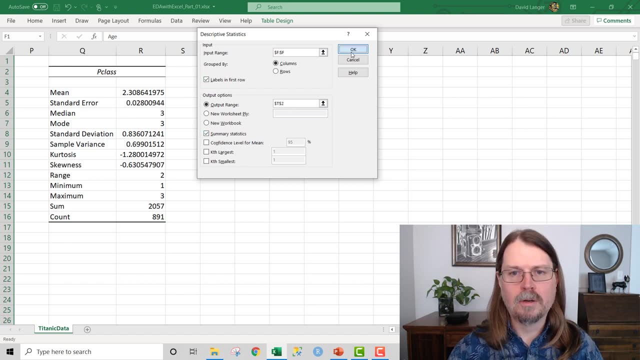 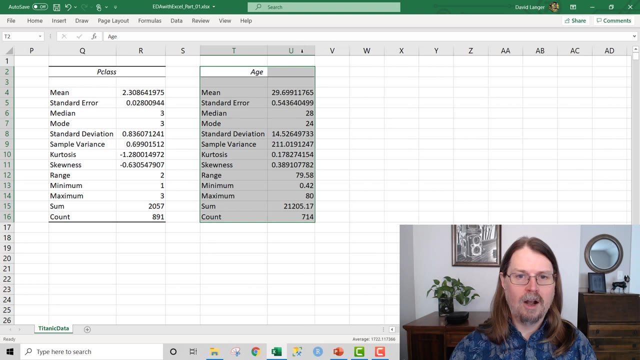 statistics and we're going to swap out column F for column C And then let's go ahead and put our t cell t2.. Okay, We'll keep everything else the same, right? We want our summary statistics and we know we have a label in the first row. Boom, Okay, Now this, this, this is cool, right? This is where. 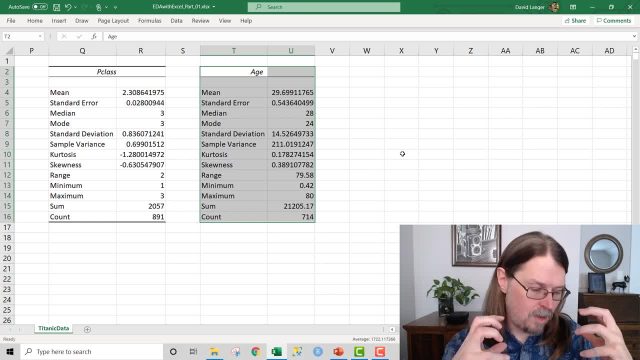 this is where the analysis tool pack really starts coming into its its own and helping you understand, helping you explore columns of numeric data. So here we have the age column and notice that it's not 891. That tells us that we're missing data, and we're missing quite a bit. 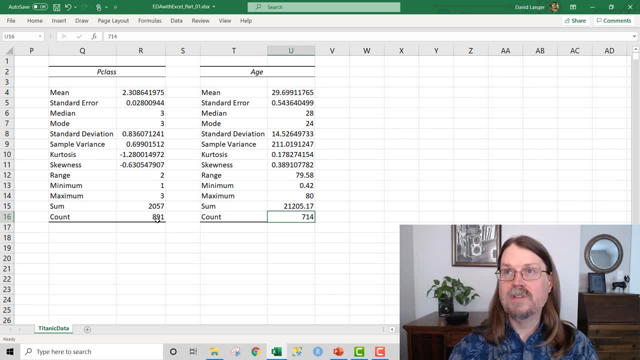 because you know so, we have 891 total rows of data in, as verified by the count here, And we can see that for p-class anyway, because p-class has no missing values, but we can see here we have 714.. So we're missing well over what? 170 rows of data. Uh, 177 rows of data, Yeah, 177. 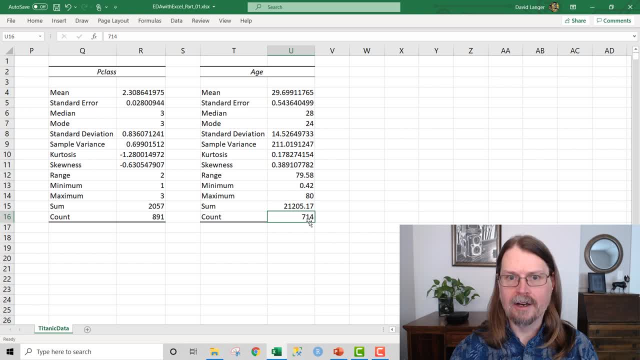 rows of data, So we're missing a lot of data here in the age column. That's the first thing that this tells us, which is problematic because missing values and when you're doing business analytics are not uncommon And unfortunately, typically there's no way for you to rectify them, because if they're, 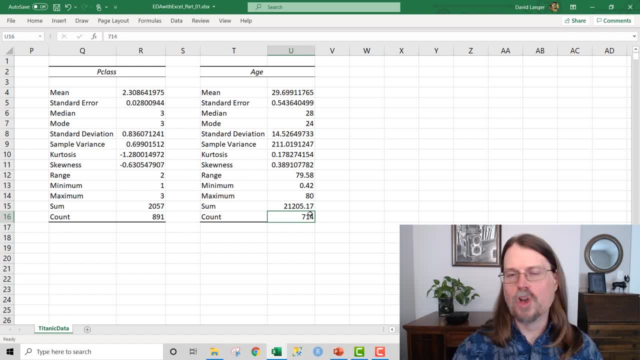 not in a database, or they're not in a computer system, or they're not in a spreadsheet. there's no way for you to go out and collect the information. So this is super interesting. Now, what we can see here is more of a typical kind of situation that you see with numeric data in 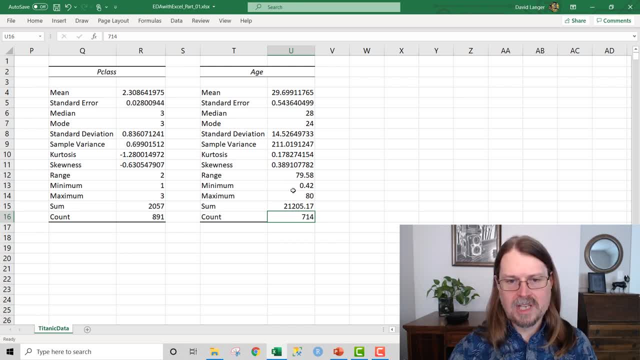 business analysis, which is we've got a range of values. Notice how our minimum age is 0.42.. So we'll assume that that's in years, obviously because of the name of the column, And maximum is 80. And then we can see the range is pretty high. And then what we can see here is like our 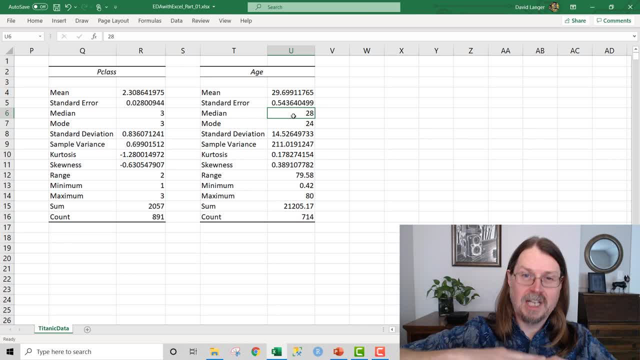 median age, which is like, if you take all 714 age values, the median is, and you arrange them in a row, right from lowest to highest, the one that's right in the very center, the 50th percentile, the halfway point in that sorted list of numbers, that's the median, which is 28.. And the most, 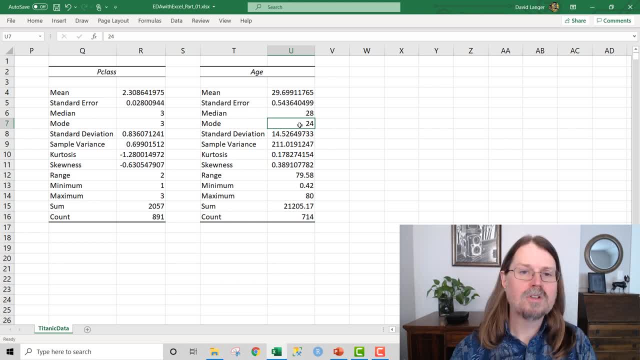 frequently occurring value is 24 years of age, And notice that we now can calculate a mean- that's probably, excuse me, a mean or an average. That's just a fancy way of saying the average which is interesting, which is 29.669, or, excuse me, 29.699 years of age. 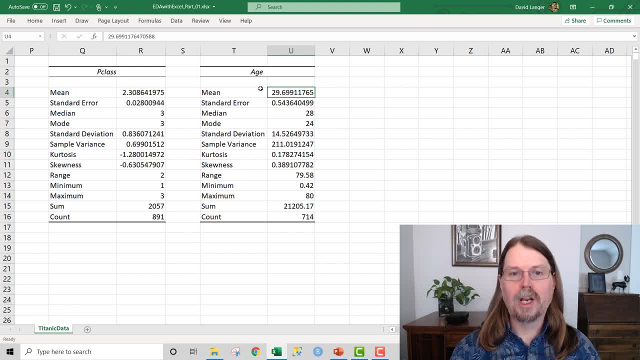 We're going to explore this in a later video, probably video three, using a histogram, which is a data visualization that you use for numeric data to kind of understand what's going on with the range of values. But this is a good first step. It tells us a lot. It tells us that: 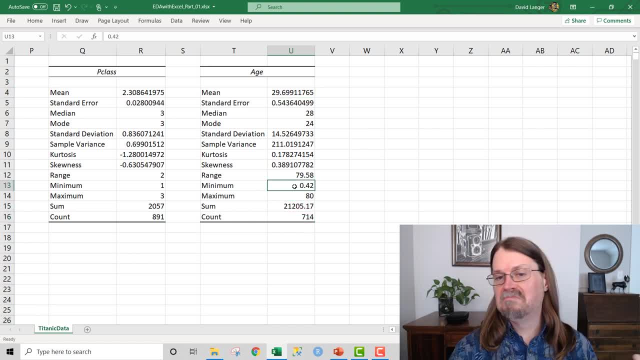 we're missing quite a bit of data. We've got ages ranging from less than a year old all the way up to 80 years old, And we've got some measures of like. well, if, prototypically, you know, if we just had to guess about the age of a passenger, we'd be able to do that, But if we 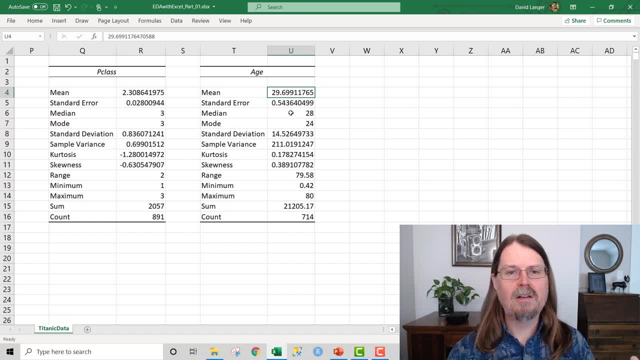 just had to guess about the age of a passenger in the Titanic, what would we guess based on the data that we have? And we would say: well, they're probably in the range of, you know, 28 to 30 years old or so on average, And a lot of folks around 24 years of age run the Titanic. as, based on the 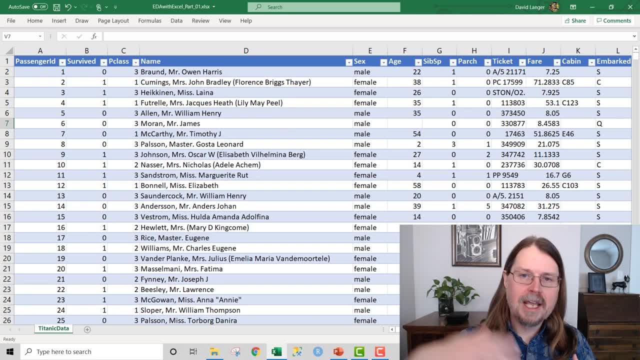 data set that we have. What I would encourage you to do is go to the GitHub and grab the files, grab the Excel files and perform this analysis on the SIBSPA and PARCH and FAIR columns- because those are the remaining numeric columns- and look for the kinds of things. 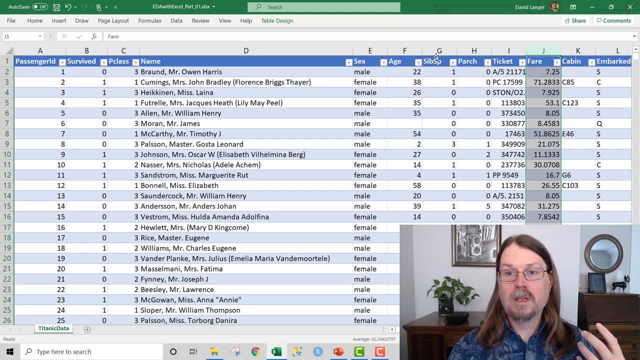 that I looked at, For example, is this really a numeric variable? Is this really a numeric variable? Because notice that pclass, for example, when we looked at that, wasn't actually a numeric variable. It was actually a categorical variable, just encoded with numbers. So we always want to. 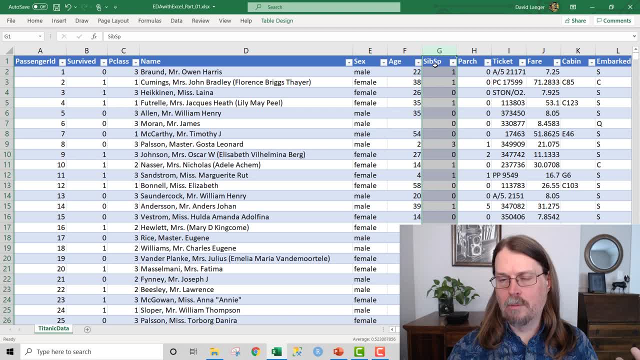 be cognizant of that. for SIBSPA, that's what I pronounce- it PARCH and FAIR, So I'd really encourage you to do the analysis as homework using the analysis tool. Also, this is the first video in the series When I record number two. 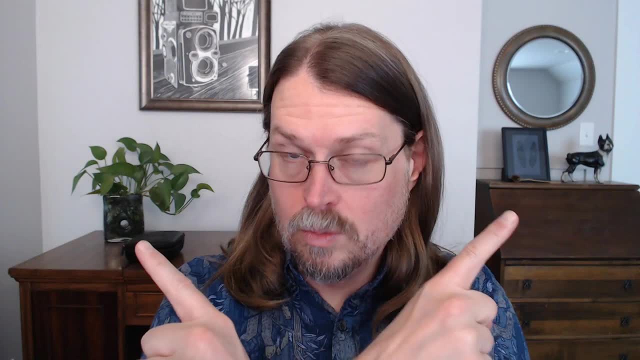 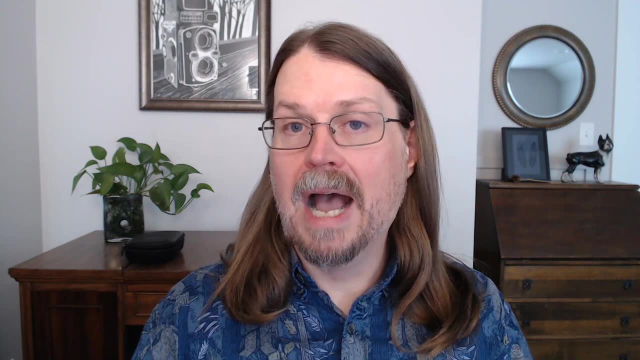 I will update the video and it will show up in one of these two places And, as I mentioned before, you can get the GitHub from the description below. And if you're interested in learning more about KPI analysis, analyzing data over time, you can go ahead and check out the video. 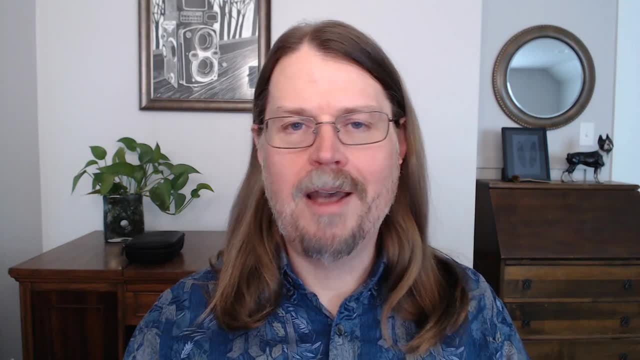 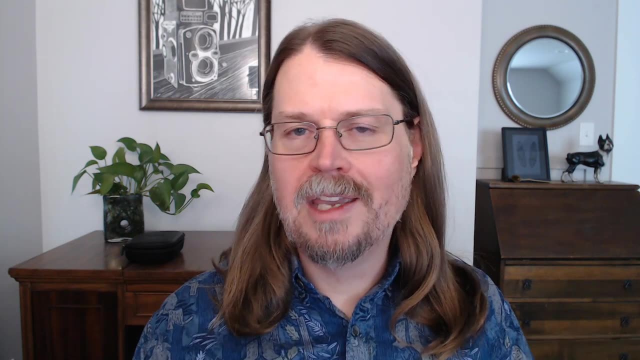 up here. It's a good time to click it now if you're interested. Okay, that's it for video number one. I'm looking forward to this series. It's going to be awesome. Until next time, please stay healthy, and I wish you very happy data sleuthing. 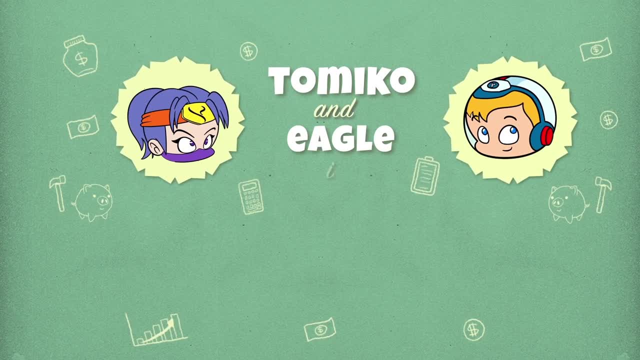 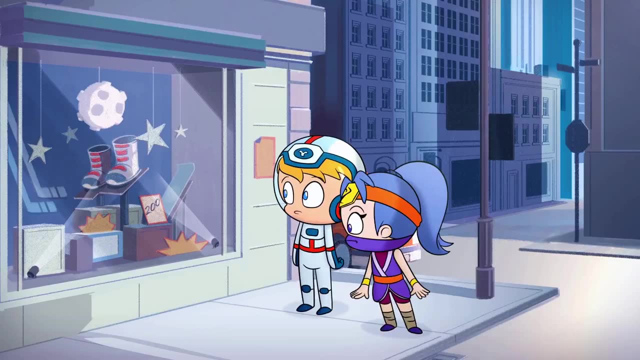 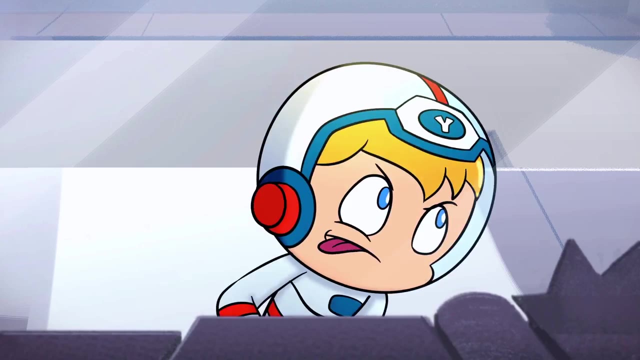 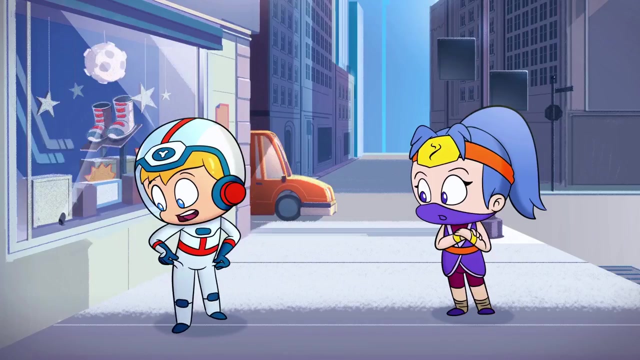 Yogotars, Tomiko and Eagle in Saving for Something Special. Wow, The new space skates are here And they're 200 bills. What's wrong? Eagle, I really want this new pair of space skates, But I don't have enough money. Hey, Tomiko, do you have some money I could borrow?